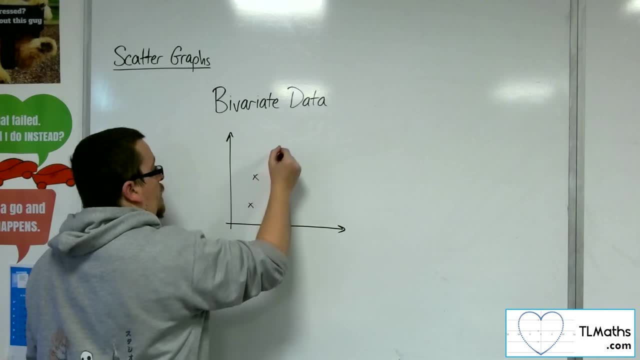 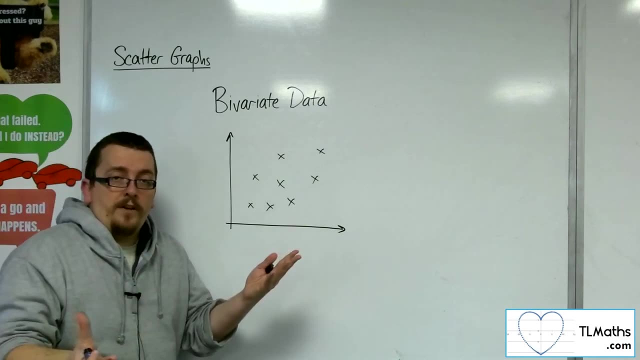 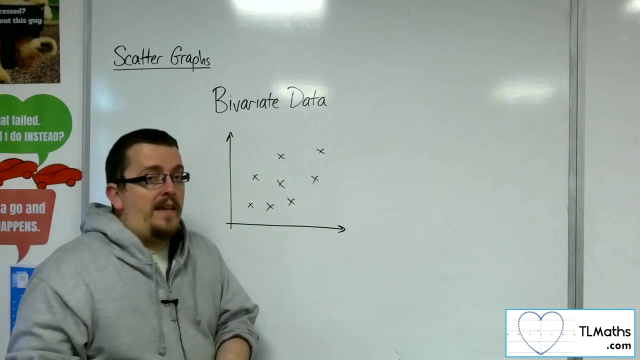 And so you would be plotting a scattergraph, okay. So this is bivariate data, okay, And what we're investigating is really all the things to do with scattergraphs that you would have learnt at GCSE, but then really extending them and pushing them forward, okay. 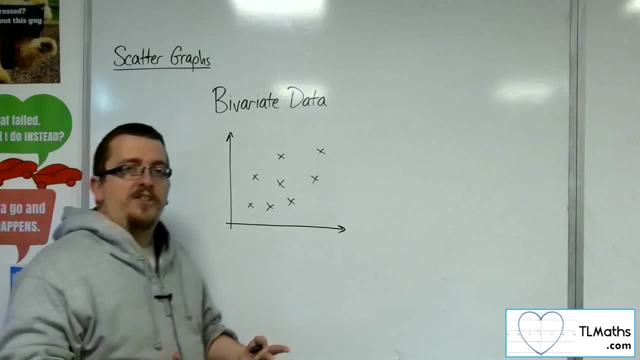 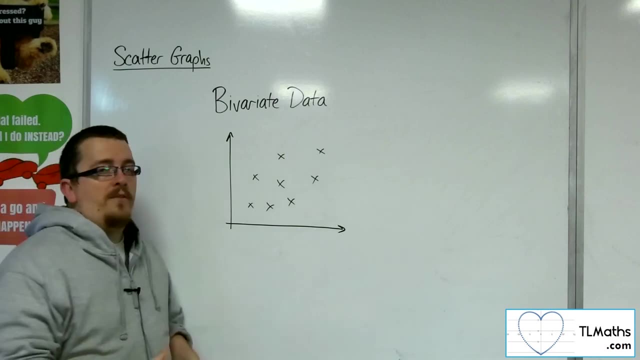 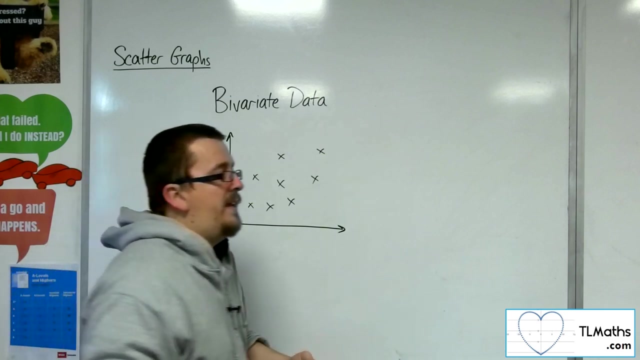 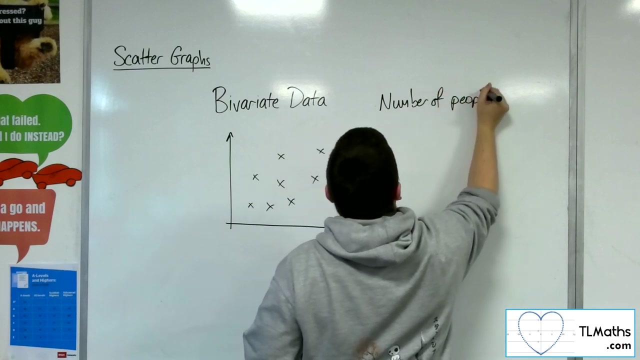 To make it a little bit more useful and to really understand what it's showing you a bit more. So one thing that's key with bivariate data is understanding how you draw it. So if you have two variables, okay, let's say let's come up with a problem. Let's say we're looking at the number of people in a lift- okay, 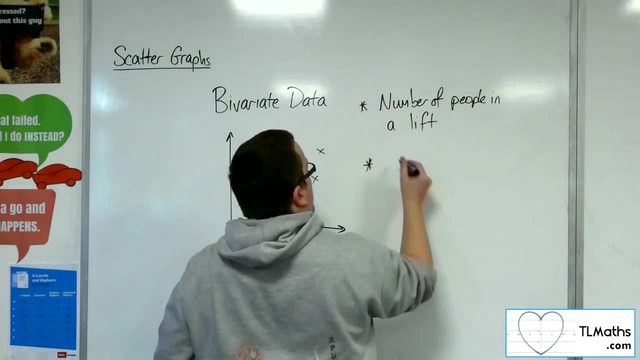 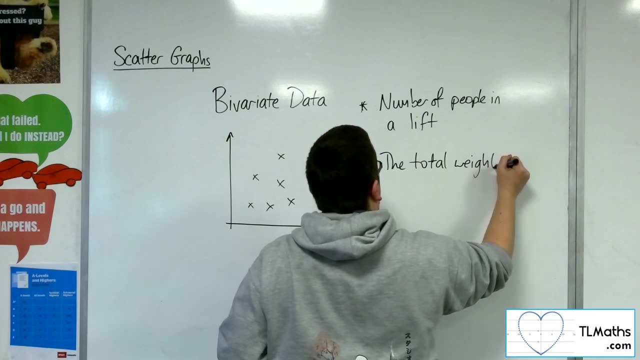 Okay, that's the number of people in a lift. Okay, that's the number of people in a lift. Okay, that's the number of people in a lift. Okay, that's one variable. And the second variable is the total weight- okay, of people in the lift. 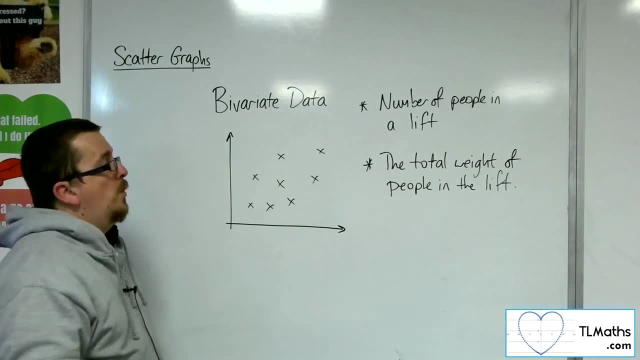 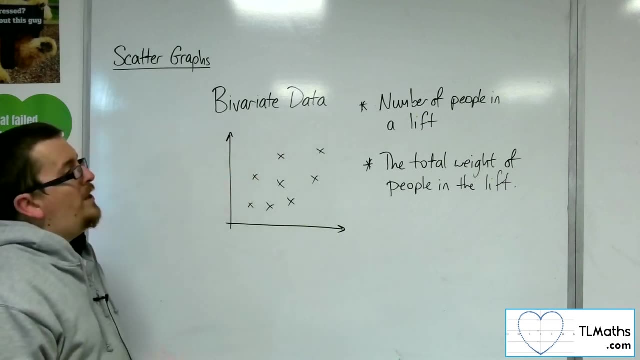 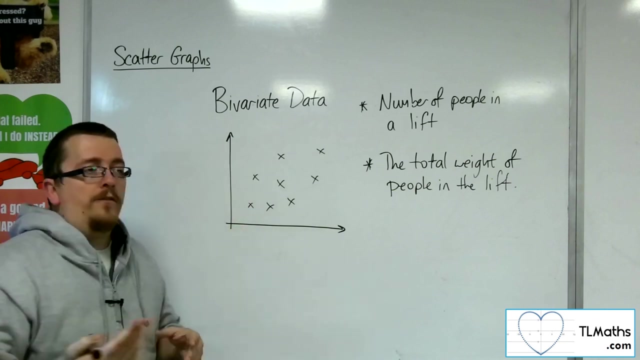 Okay, so they are the two variables. So when you're plotting a scattergraph, So when you're plotting a scattergraph, which one of these should go on your horizontal x-axis and which one should go in the vertical y-axis, You might be thinking, well, it doesn't really matter, okay. 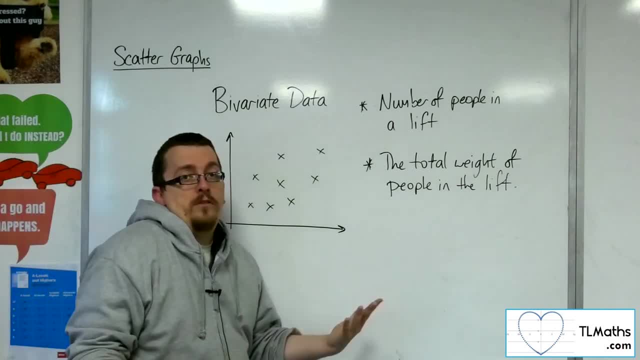 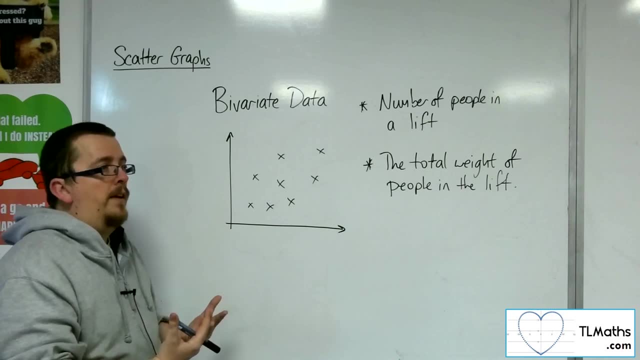 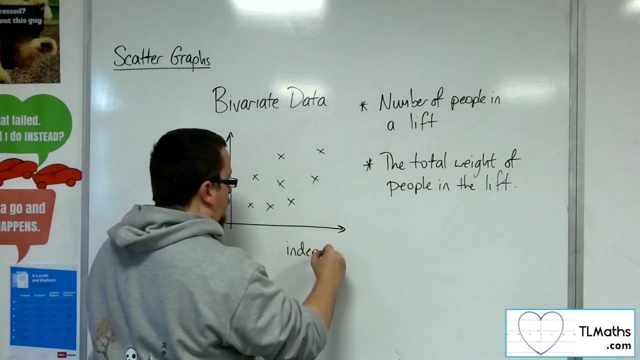 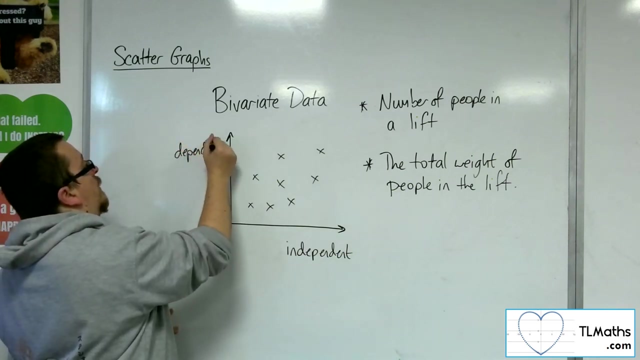 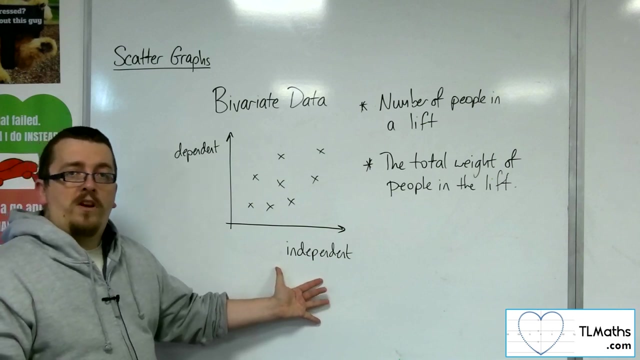 And in some cases that's true, But there is a generic concept that goes with this: That the horizontal axis should be the integral, That the vertical axis should be the independent variable, While the vertical axis should be the dependent variable, And what that means is that this variable is independent of the other and does not rely on the other, while this one depends on this variable. okay, 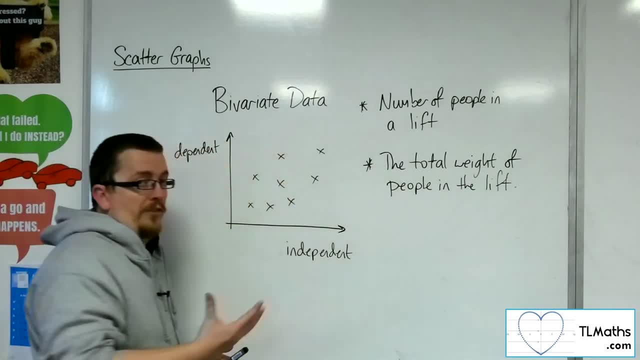 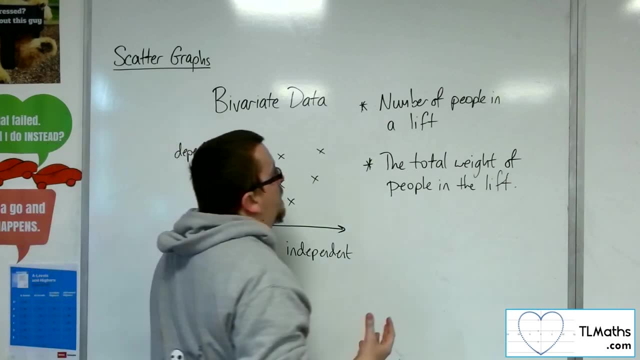 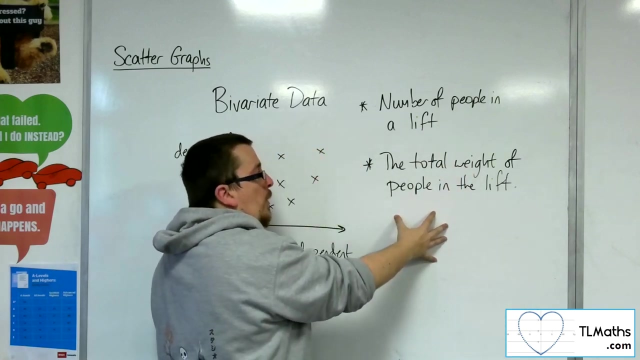 So this in context problems is usually quite straightforward to figure out Which one should be which. So does the number of people in the lift depend on the total weight, Or does the total weight depend on the number of people in the lift? 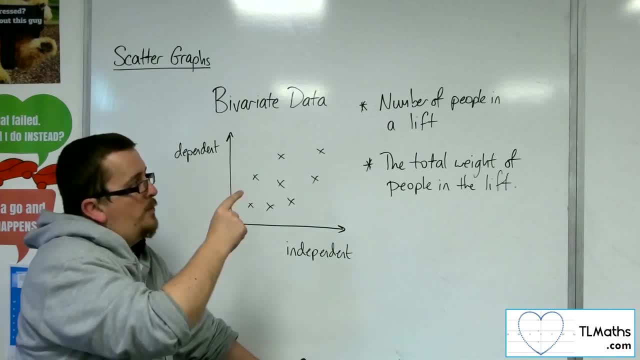 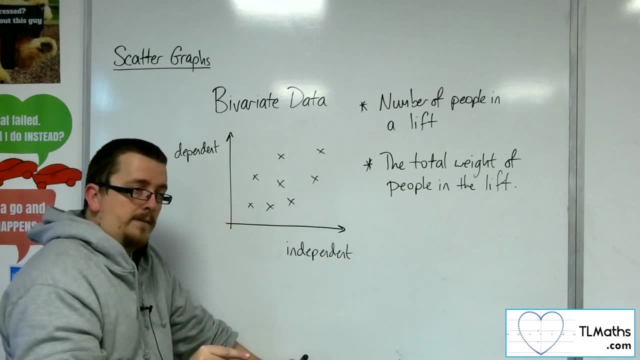 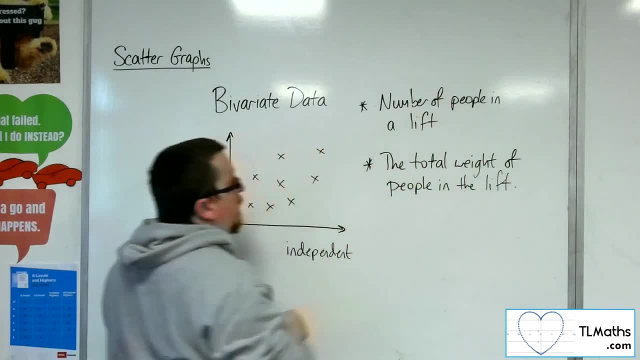 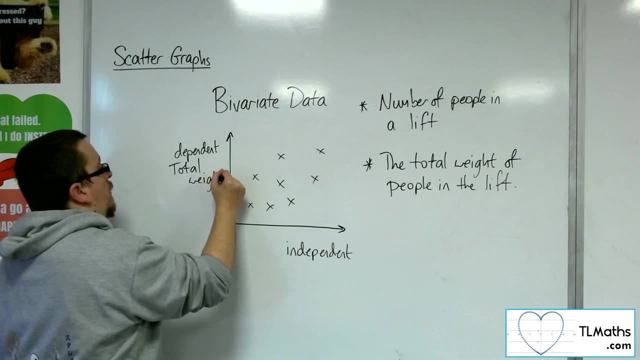 The total weight will depend on the number of people in the lift. The total weight will depend on the number of people in the lift. The total weight will depend on the number of people in the lift. number of people in the lift. So the total weight is the dependent variable, while the 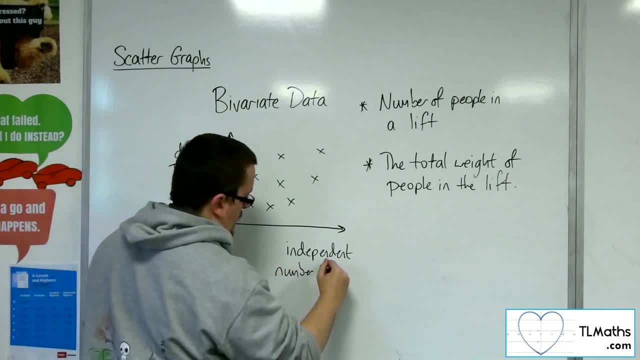 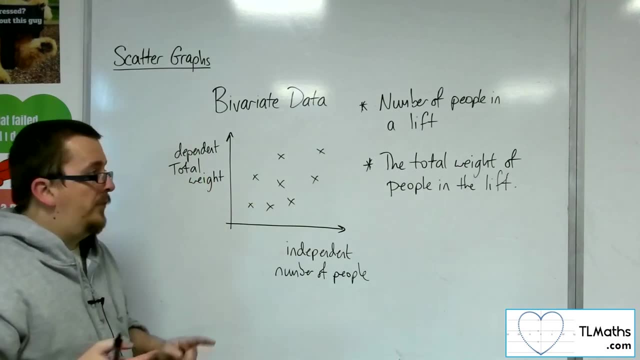 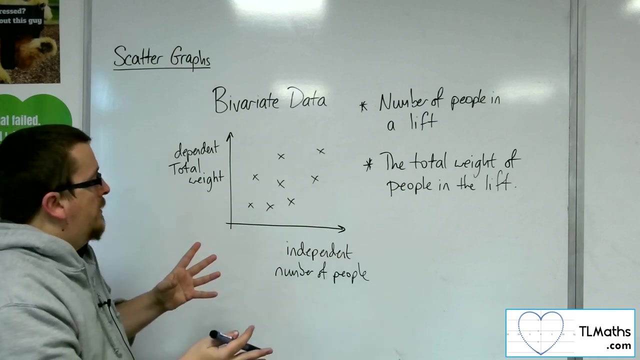 number of people in the lift is the independent variable, And so you should plot number of people along the x-axis and total weight of the y-axis. So that is how you would generally do it. So another way to think of the independent variable is the one that you have some control. 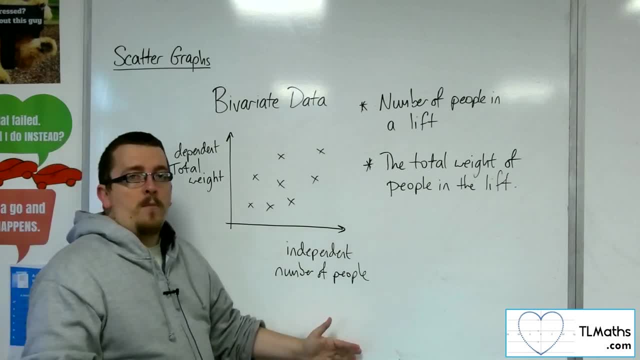 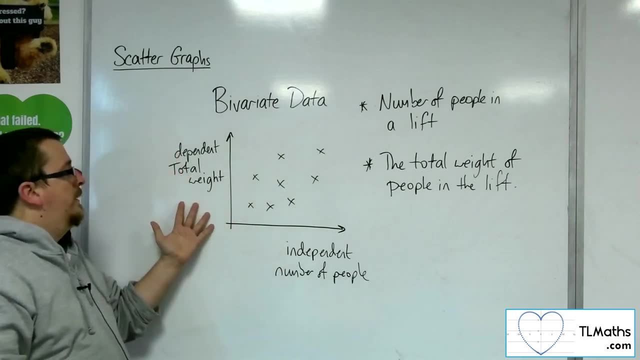 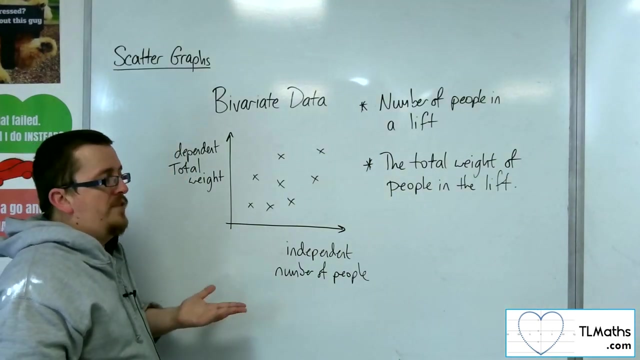 over. I have control over the number of people that are going into the lift, for example. That is something that I could control, Whereas their total weight I have no control over. Now in some cases, if I just gave you a set of numbers with no context whatsoever and 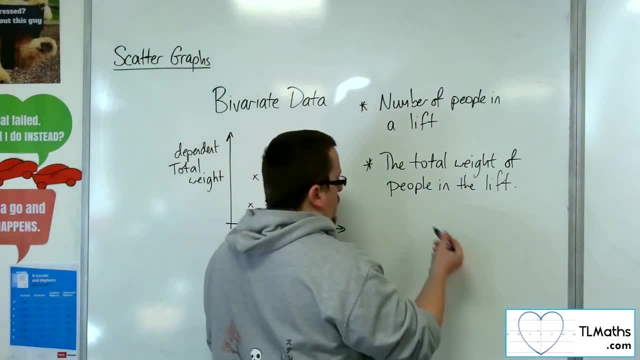 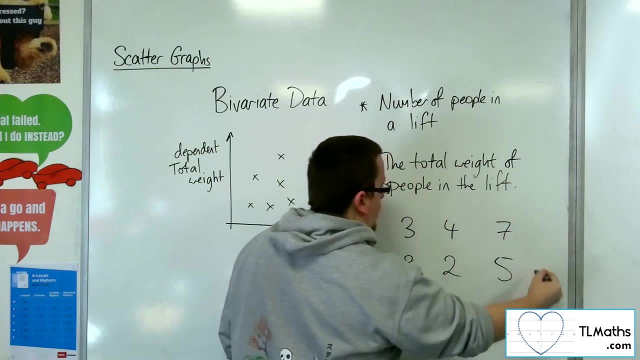 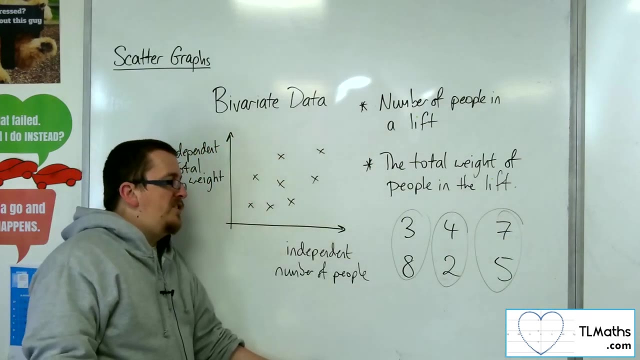 I said, If I plot these numbers, so 3,, 4,, 7,, 8,, 2,, 5, and plot these as pairs of numbers, as coordinates, then there's no kind of nothing telling me which is the independent and which. 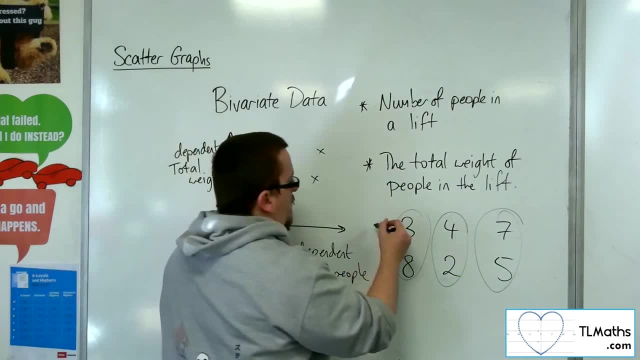 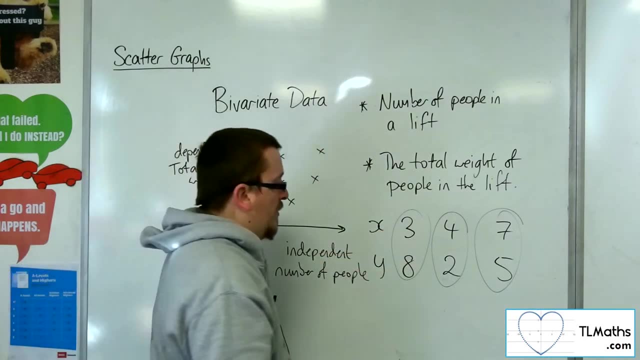 is the dependent variable here. So really I could treat either those as the x's and those as the y's, which might be the natural way of thinking about it, because I've got those on top and those at the bottom, But it would be just as equivalent to really. 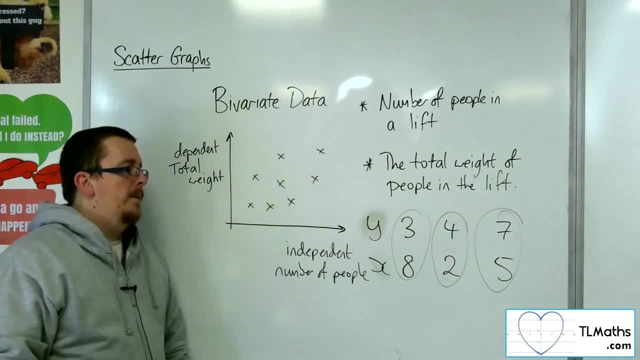 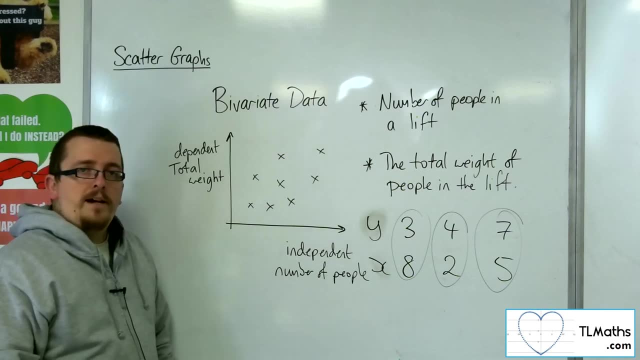 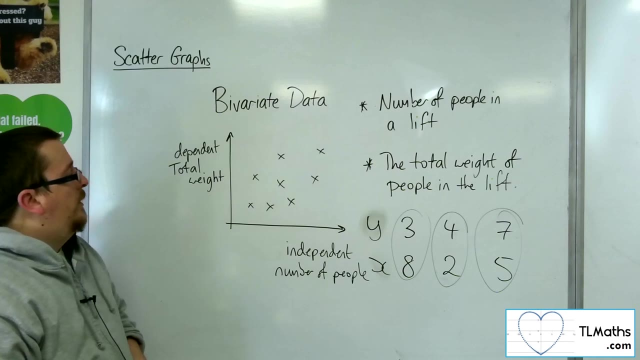 say: well, they could be the x's and they could be the y's. It will have an effect upon some of the things that we consider in this set of videos, But just so that you're aware, in the context of problems, that there is a difference between independent and dependent. 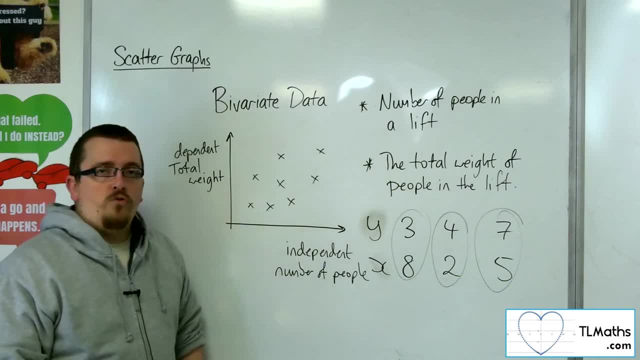 variables. Generally, the independent variable is drawn on the x-axis. 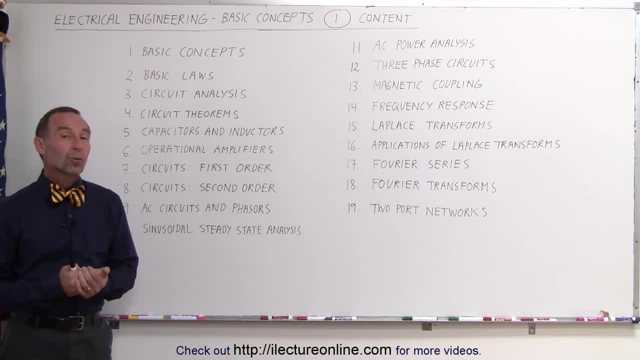 Welcome to Electro-Online. In this video, we're going to show you what is coming up in this particular series. We're going to be talking about electrical engineering. There's a lot of topics to be covered. These are basically the 19 chapters that we're going to cover, starting with some. 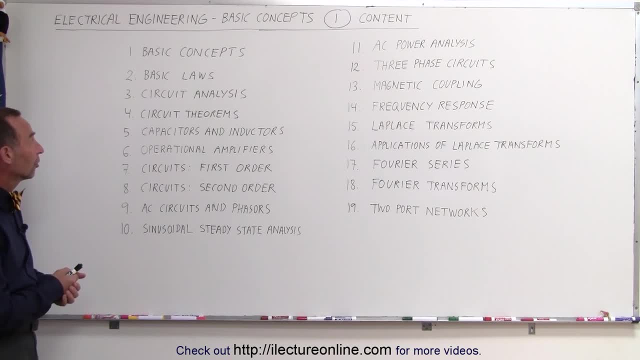 basic concepts. then the basic laws of circuits, some circuit analysis, the basic concepts of circuit analysis. then we'll get into some specific circuit theorems. We'll talk about capacitors and inductors in circuits, operational amplifiers, also known as op-amps, We'll talk about 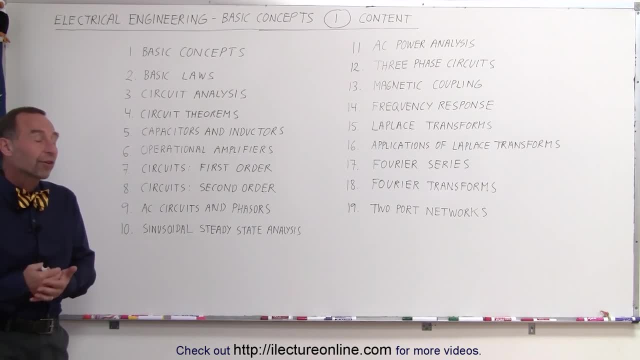 circuits that can be solved using first order techniques, so first order differential equation techniques and circuits that will require second order differential equation techniques to be solved. We'll talk about AC circuits and phasors. so we'll talk about phasor diagrams and the 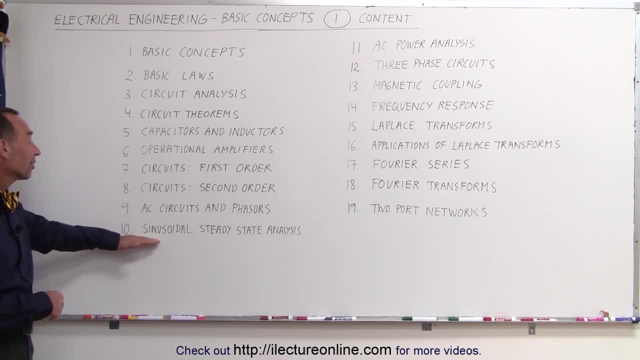 difference in phase between the current and the voltage. We'll talk about sinusoidal steady state analysis. so we'll do circuits with steady state analysis. so we'll do circuits with steady state conditions in the circuit. Then we'll talk about AC power analysis. We'll then talk about 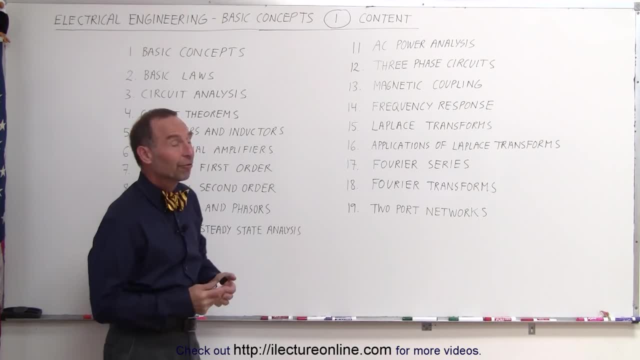 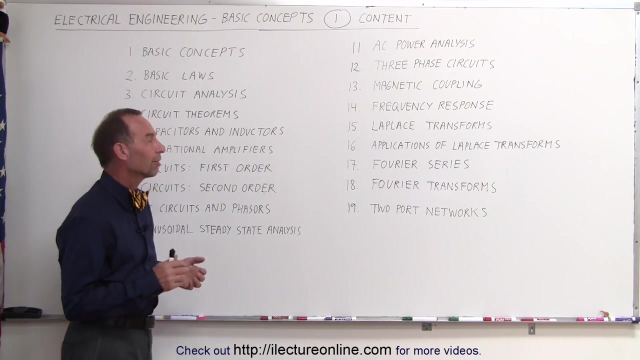 the three phase circuits, magnetic coupling, frequency response, and then, finally, we'll get into the more difficult concepts such as Laplace transforms, applications of Laplace transforms, Fourier series, Fourier transforms and finally, two-port networks. So a lot of material, that's. 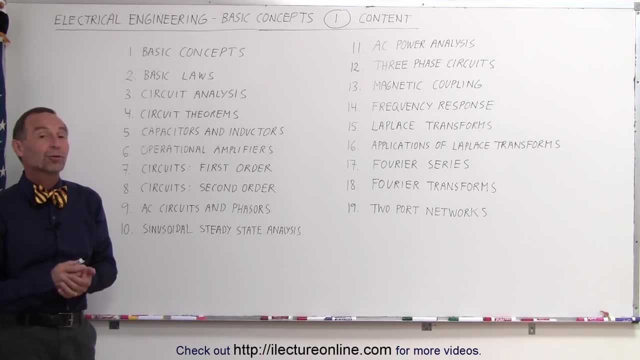 coming up. I've had some requests to do: Laplace transforms, Fourier series, Fourier transforms and so forth. I figured this is a good place to put them in a course of electrical engineering. Hopefully you'll enjoy these. Stay tuned and we'll get started on number one.